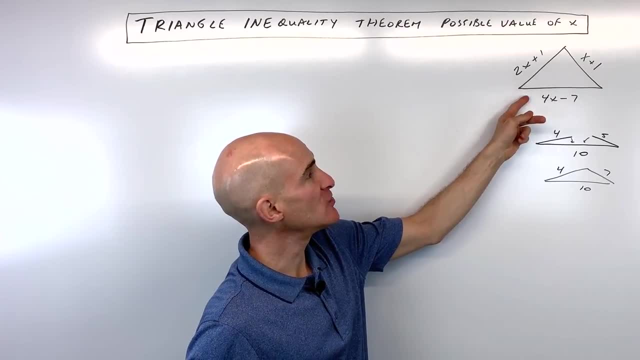 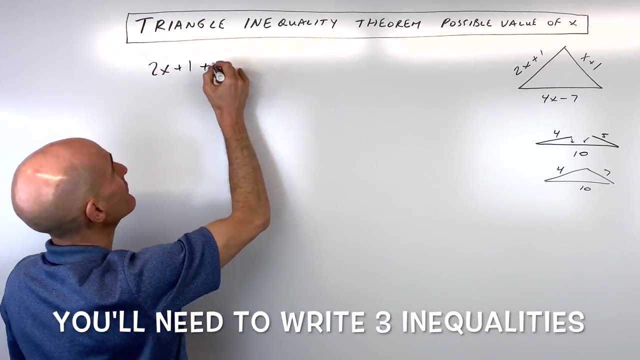 What you would do in this algebraic example is you would take any two sides- say, for example, 2x plus 1 plus 4x minus 7, has to be greater than the third side, which is x plus 1.. 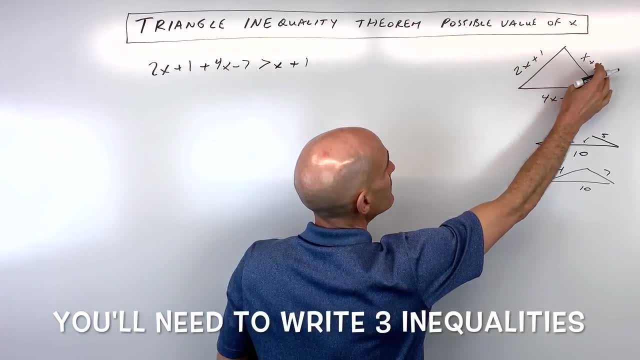 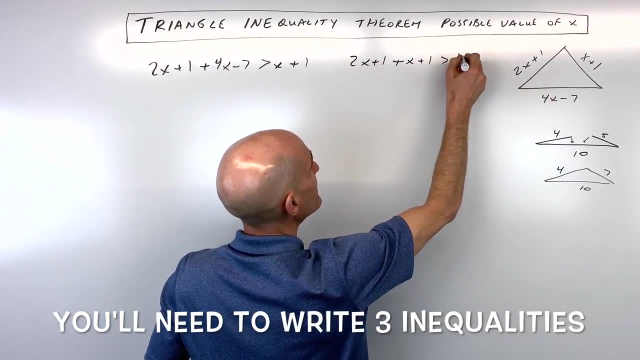 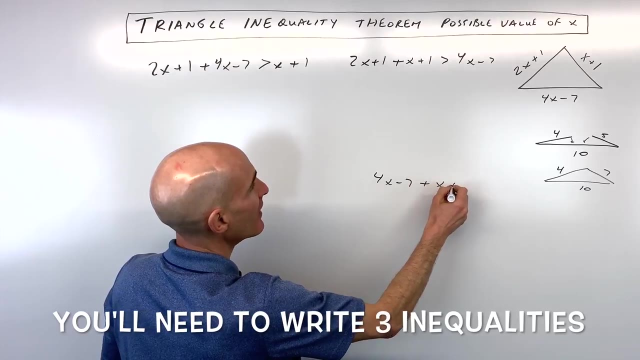 So you would do this. But we also have to take into account that 2x plus 1 plus x plus 1, those two sides have to be greater than 4x minus 7.. And also we have 4x minus 7 plus x plus 1: has to be greater than 2x plus 1.. 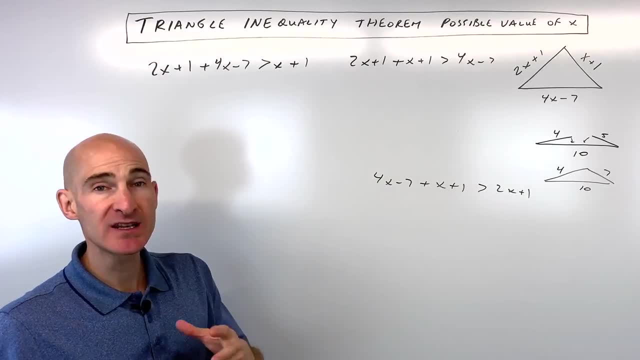 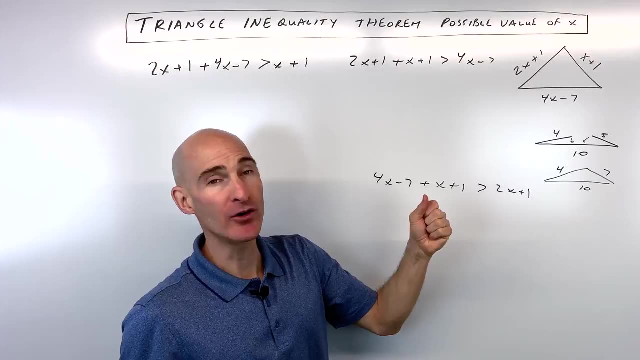 Okay, so what we're going to do is we're going to solve these three inequalities separately and then we're going to take a look at the solutions on the number line to find out what the possible values are, What the possible values of x are, in order to make this a true triangle. so a possible triangle that you can draw. 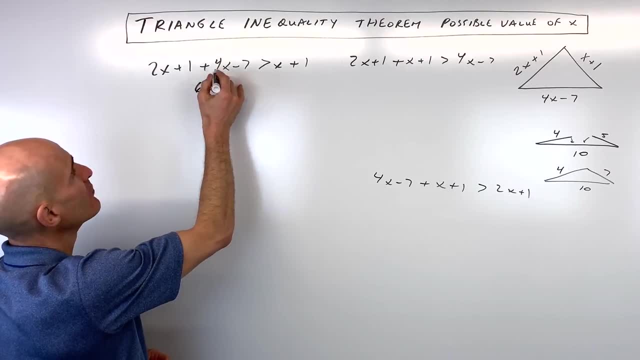 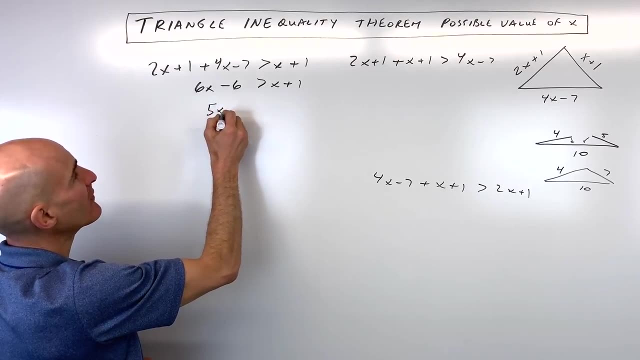 So let's go ahead and solve this: 2x plus 4x is 6x, positive 1 and negative 7 is negative 6.. And here what I'm going to do is I'm going to subtract x from both sides, so that's going to be 5x. 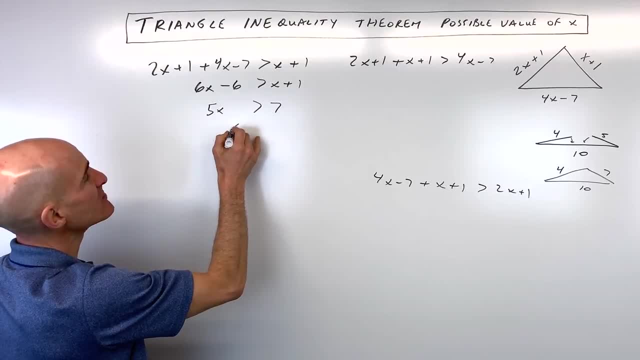 I'm going to add 6 to both sides. that's going to give us 7.. And if we divide both sides by 5, you can see that x is going to be greater than 7 fifths. So that's one constraint. 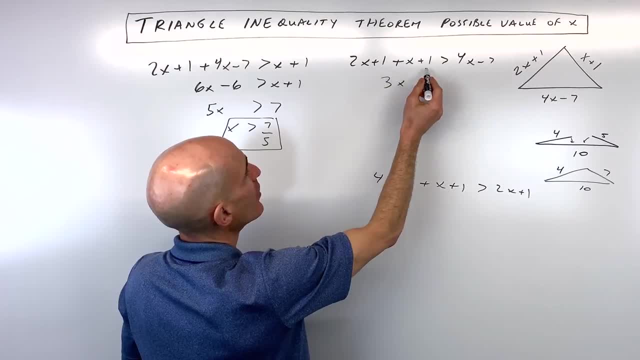 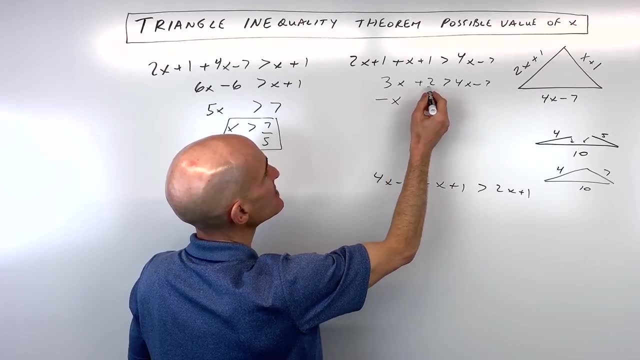 Now over here we're going to solve. this gives us 3x. 1 plus 1 is 2.. Here, if I, let's see, subtract 4x, that's going to be negative 1x. If I subtract 2 from both sides, that's going to give us negative 9.. 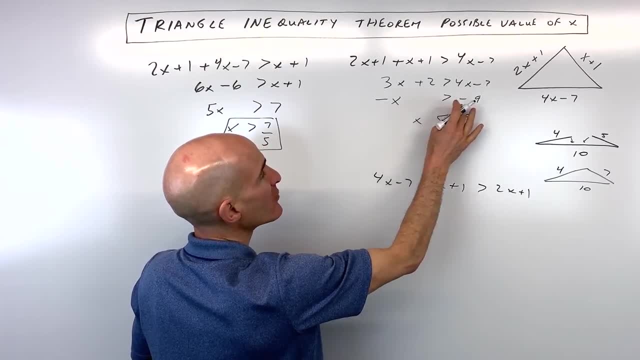 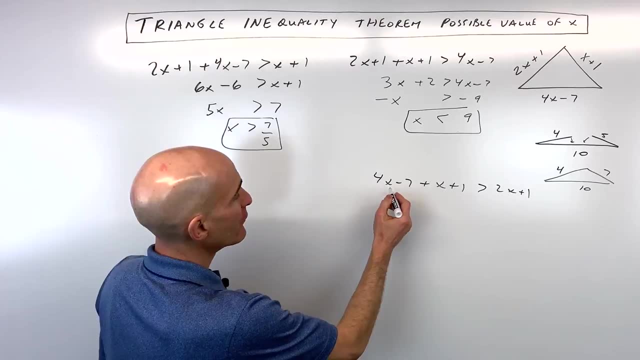 If I divide both sides by negative 1, whenever you multiply or divide both sides by a negative number, the inequality sign flips or changes direction. And then the third inequality we have: 4x plus 1x is 5x, Negative 7 and positive 1 is negative 6.. 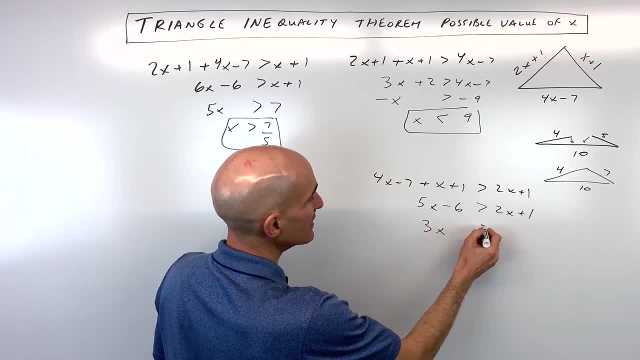 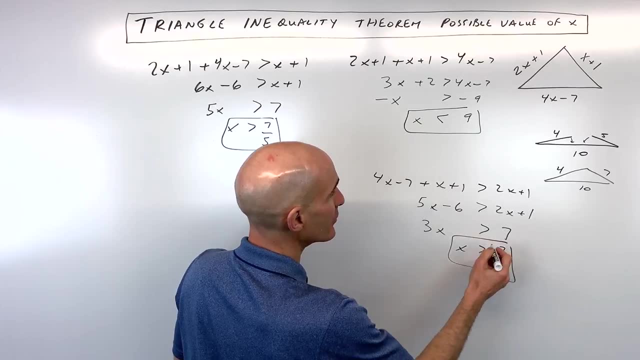 Here: if I subtract 2x from both sides, we get 3x, And if I add 6 to both sides, we get 7.. If I divide both sides by 3 to get x, by itself we have. x is greater than 7 thirds. 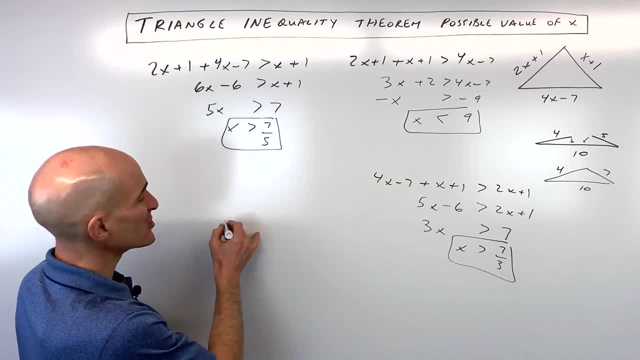 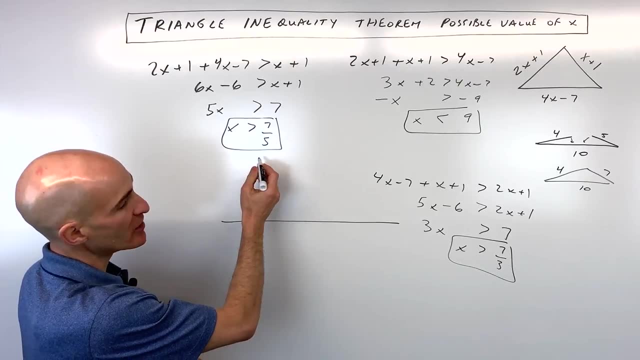 So I think that part you're probably pretty familiar with. But this part here is what tricks students a little bit. What you want to do is you want to plot these on the number line from lowest to greatest. So the smallest number here looks like it's going to be 7 fifths. 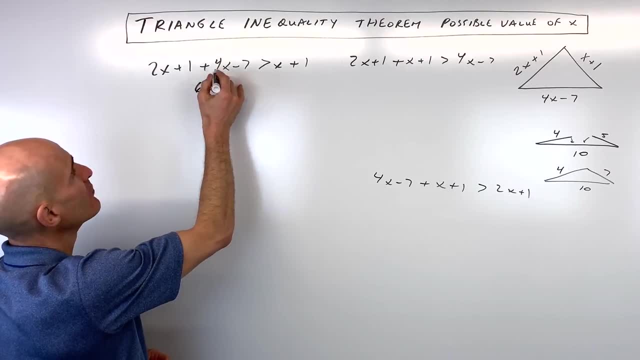 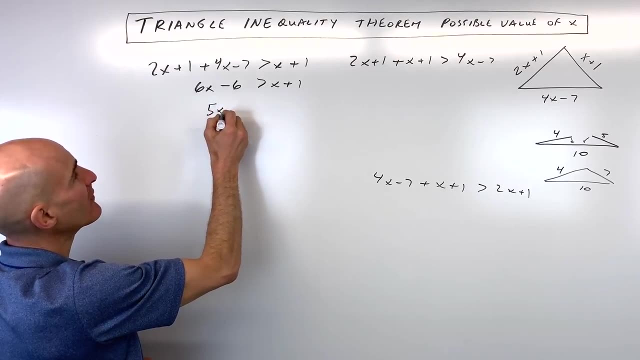 So let's go ahead and solve this: 2x plus 4x is 6x, positive 1 and negative 7 is negative 6.. And here what I'm going to do is I'm going to subtract x from both sides, so that's going to be 5x. 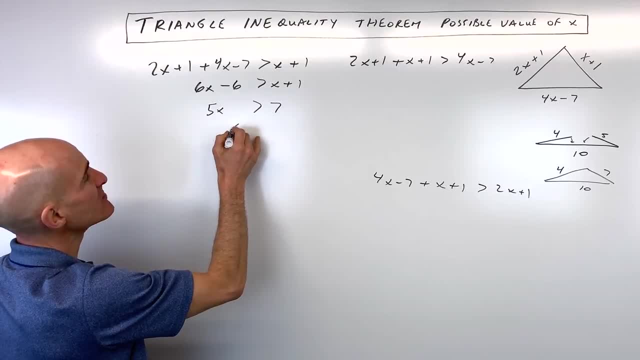 I'm going to add 6 to both sides. that's going to give us 7.. And if we divide both sides by 5, you can see that x is going to be greater than 7 fifths. So that's one constraint. 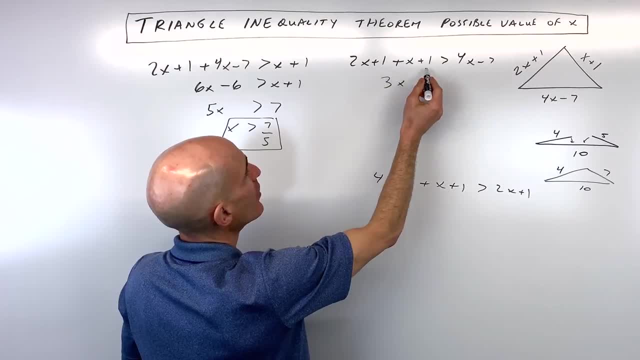 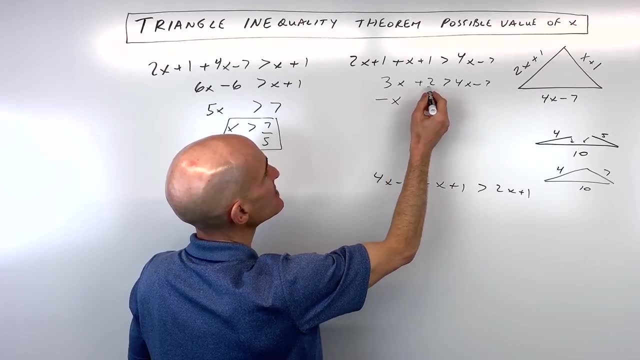 Now over here we're going to solve. this gives us 3x. 1 plus 1 is 2.. Here, if I, let's see, subtract 4x, that's going to be negative 1x. If I subtract 2 from both sides, that's going to give us negative 9.. 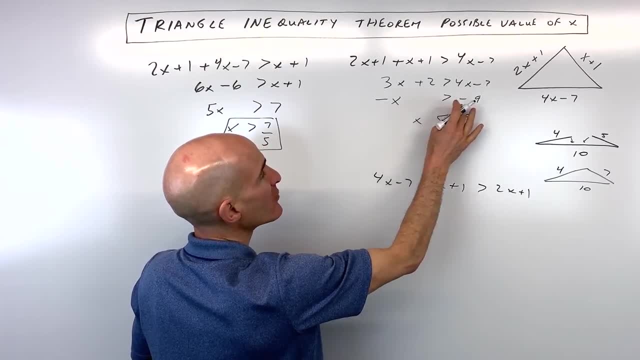 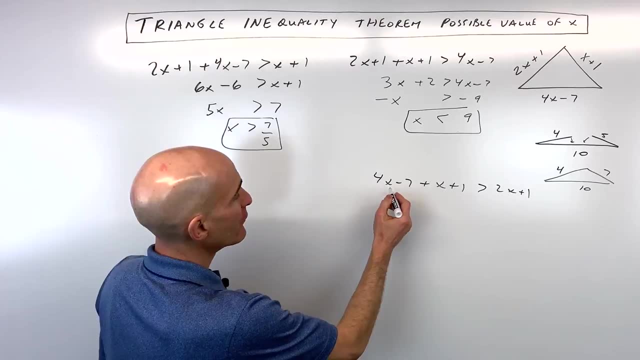 If I divide both sides by negative 1, whenever you multiply or divide both sides by a negative number, the inequality sign flips or changes direction. And then the third inequality we have: 4x plus 1x is 5x, Negative 7 and positive 1 is negative 6.. 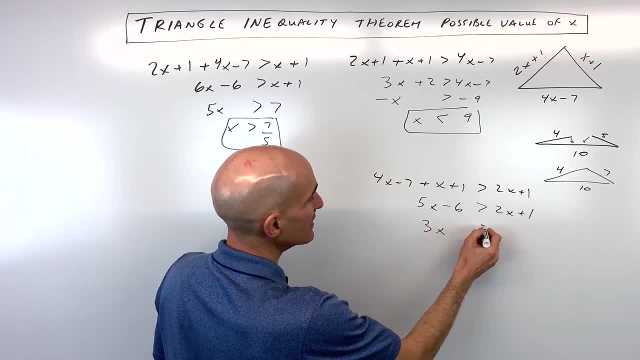 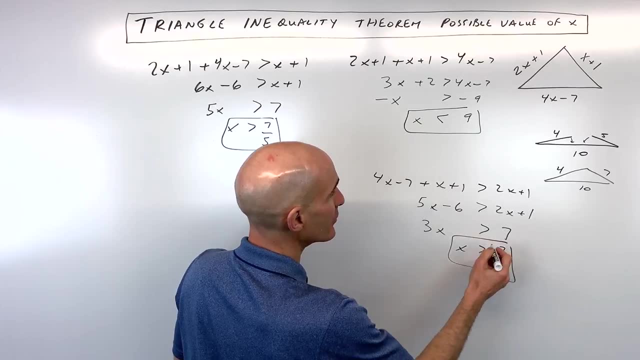 Here: if I subtract 2x from both sides, we get 3x, And if I add 6 to both sides, we get 7.. If I divide both sides by 3 to get x, by itself we have. x is greater than 7 thirds. 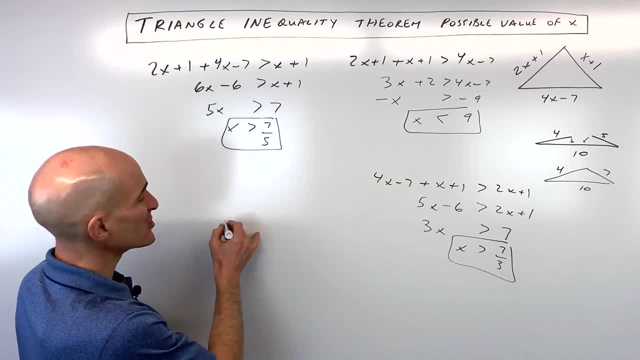 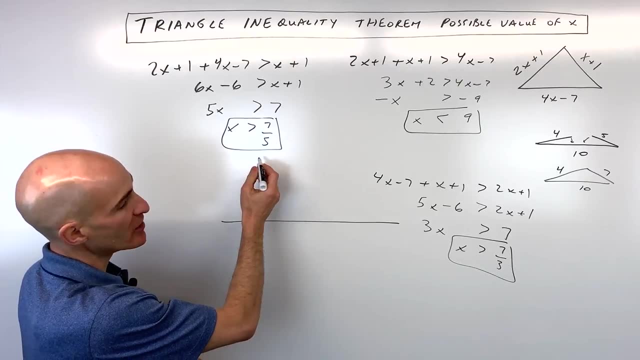 So I think that part you're probably pretty familiar with. But this part here is what tricks students a little bit. What you want to do is you want to plot these on the number line from lowest to greatest. So the smallest number here looks like it's going to be 7 fifths. 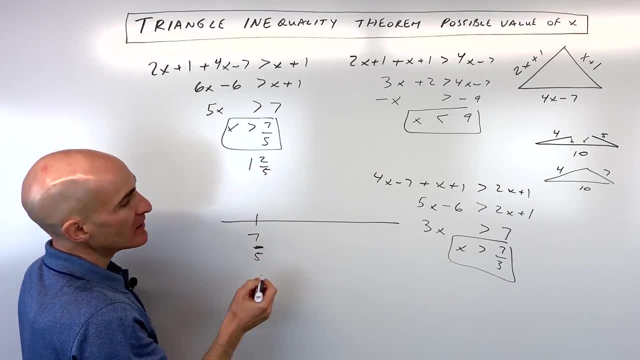 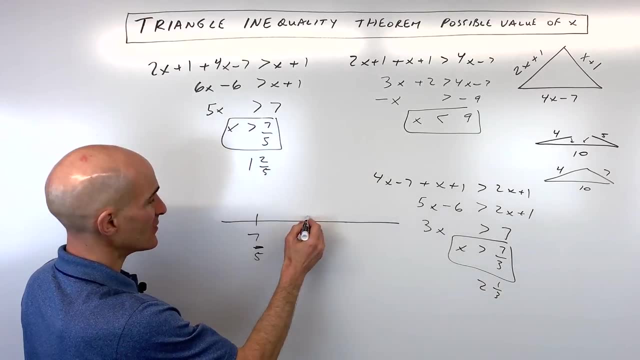 Okay, 7 fifths is like 1 and 2 fifths. Let's see, the next largest is going to be 7 thirds, which is actually like 2 and 1 third. so that's going to be right about here. let's just say 7 thirds. 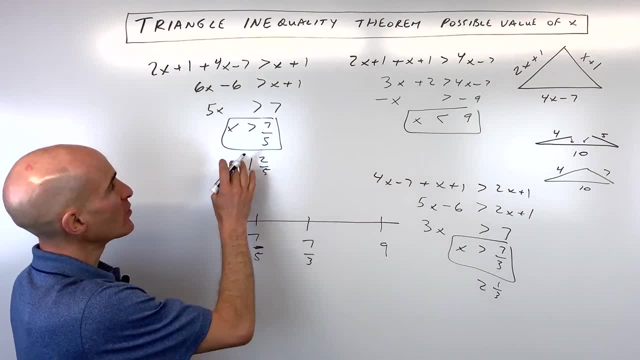 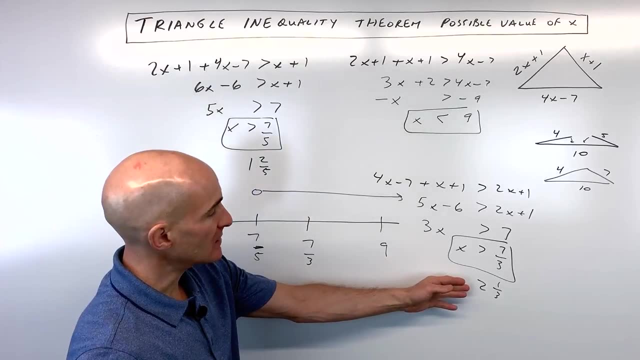 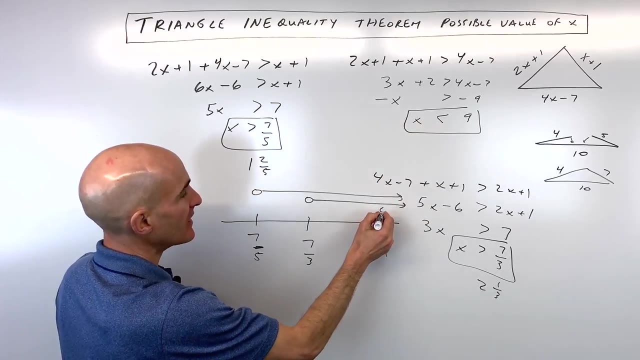 And then over here, 9 is the largest, so that's 9.. Okay, so we want x to be greater than 7 fifths, so greater than means to the right. We want it to be greater than 7 thirds, okay, and we want x to be less than 9.. 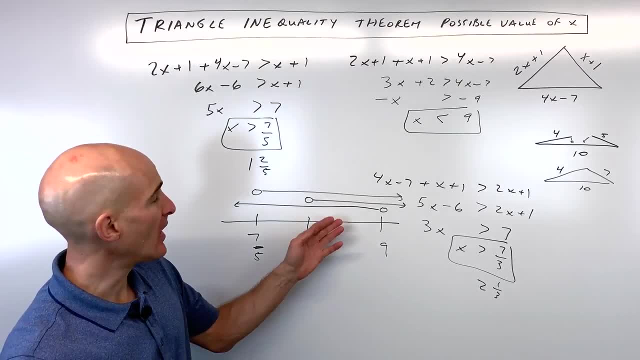 Okay, so now that we've graphed all three of those on the number line, what you want to look for is that overlapping region. So here you can see if you're over here between 7 fifths and 7 thirds, you know. 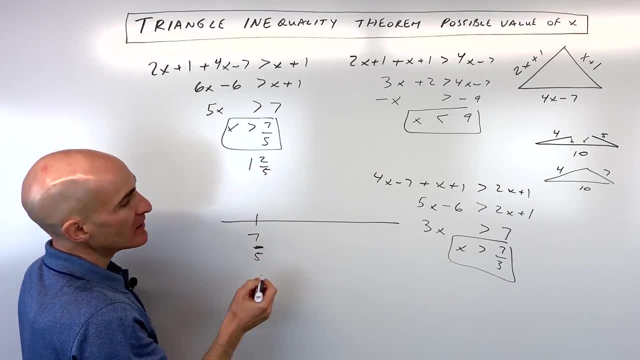 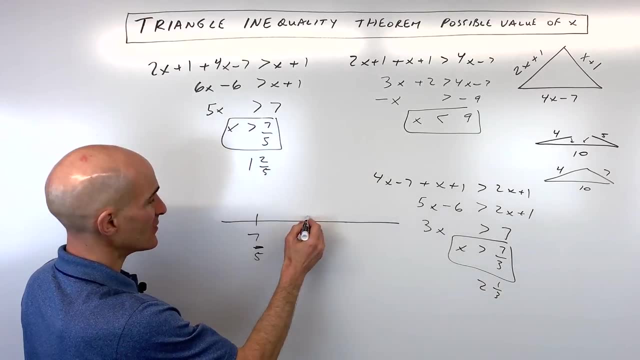 Okay, 7 fifths is like 1 and 2 fifths. Let's see, the next largest is going to be 7 thirds, which is actually like 2 and 1 third. so that's going to be right about here. let's just say 7 thirds. 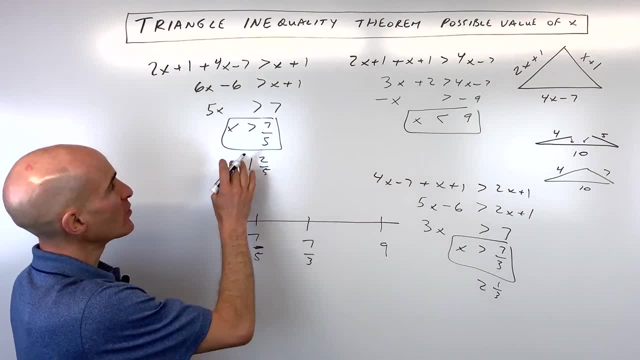 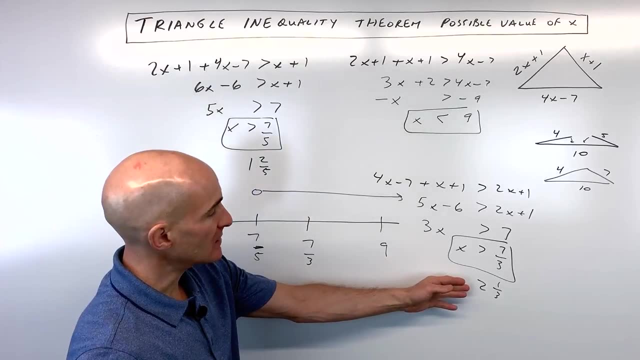 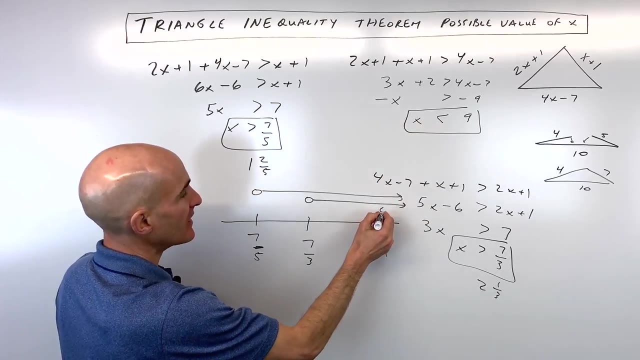 And then over here, 9 is the largest, so that's 9.. Okay, so we want x to be greater than 7 fifths. so greater that means to the right. We want it to be greater than 7 thirds, okay, and we want x to be less than 9.. 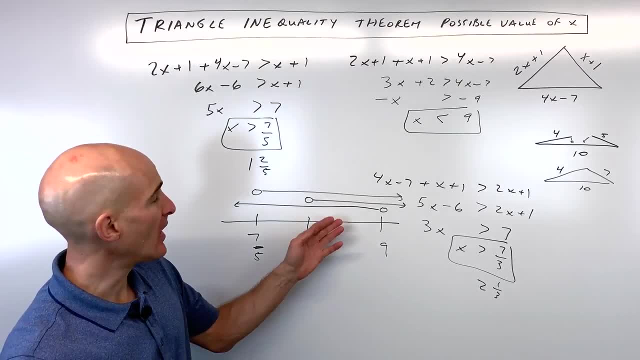 Okay, so now that we've graphed all three of those on the number line, what you want to look for is that overlapping region. So here you can see if you're over here between 7 fifths and 7 thirds, you know. 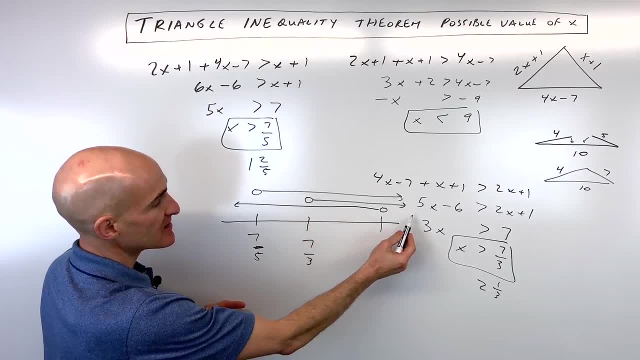 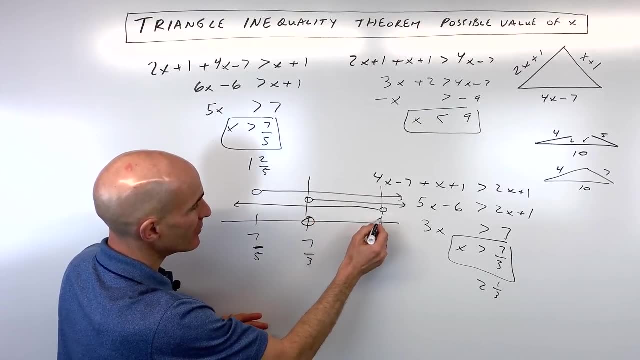 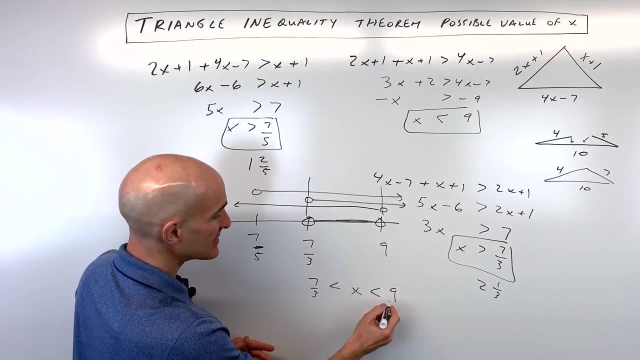 two of the constraints are satisfied, but not this third constraint, etc. So what you want to do is look at where they're overlapping, So you can see they're overlapping right here in this region in between 7 thirds and 9.. So as long as x is greater than 7 thirds and at the same time less than 9,. 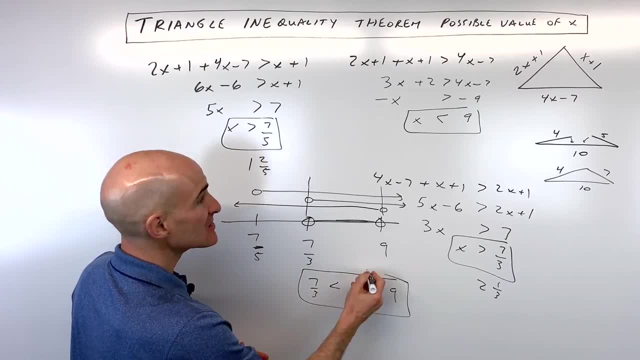 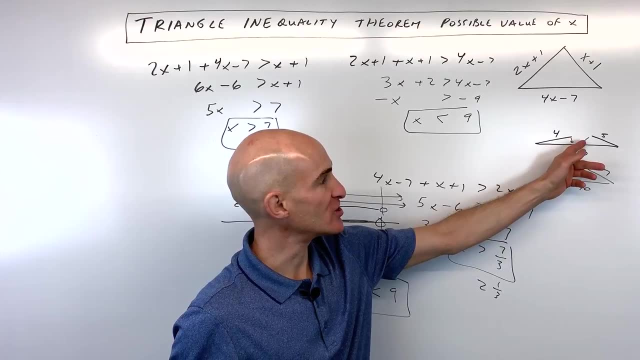 basically sandwiched in between 7 thirds and 9, then this is going to actually be a triangle that you can draw, Meaning that any two sides will add up to more than the third side. we won't have a situation here where there's a gap, etc.